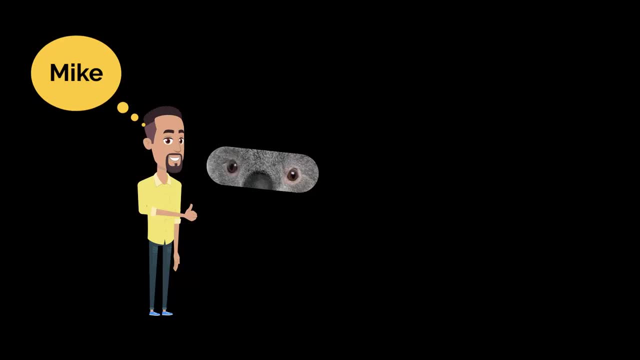 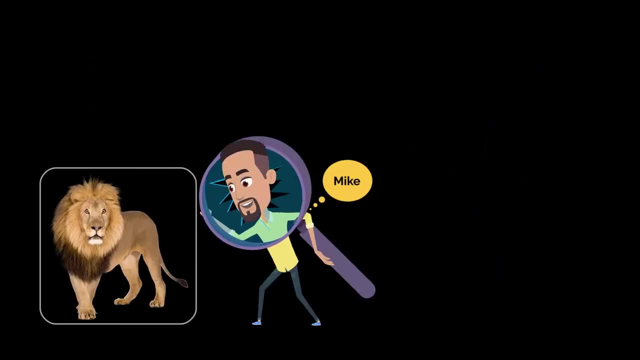 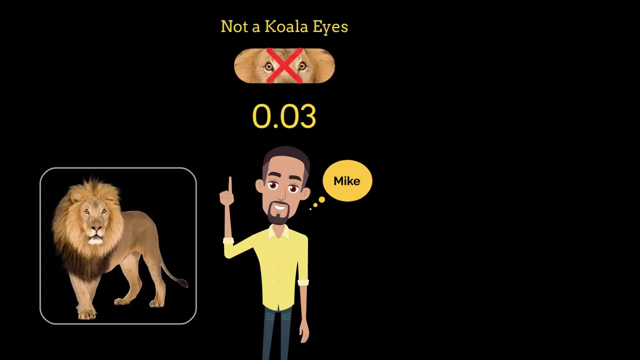 So Mike has become now expert koala eye detector. Similarly, Mohan is an expert koala nose detector. When you give them an image of a lion, Mike will say the decision is 0.03 because the eyes they are like round eyeballs but they don't look like koala's eyes. 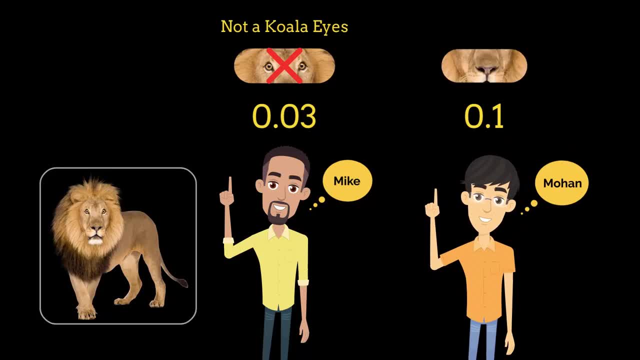 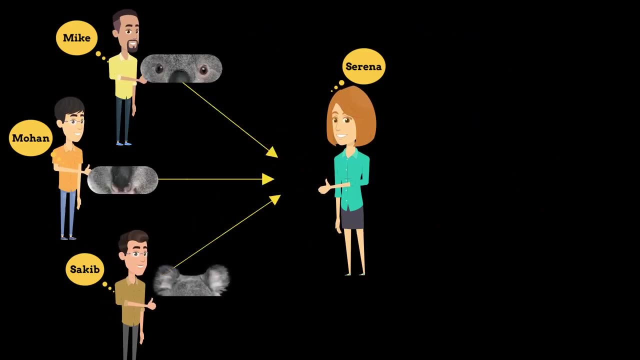 So 0.03.. Similarly for nose: he can just give some score, and if the score is more than 0.5 we'll say: yeah, those are koala's eyes or nose. You can extend this collaboration further and make Shakib an ear detection expert, And then these three students can go to Serena and Serena can work on. 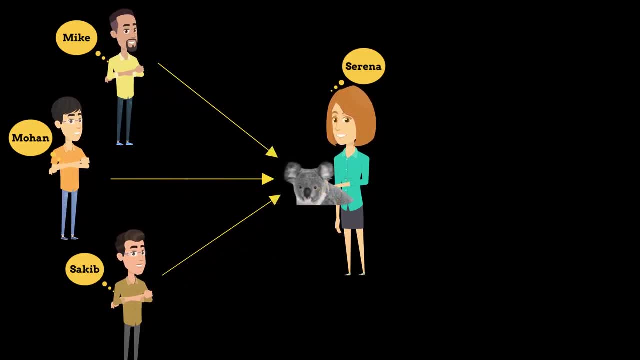 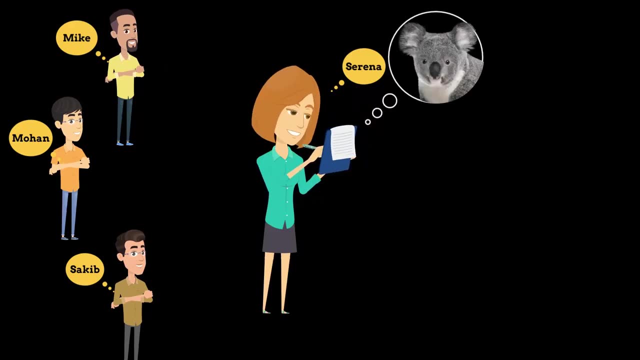 deciding if the image has koala's face or not. So once Mike Mohan and Shakib says that this image has koala's eyes, nose and ears, Serena can use their work to figure out if the image has koala's face or not, And she can use a formula like this: 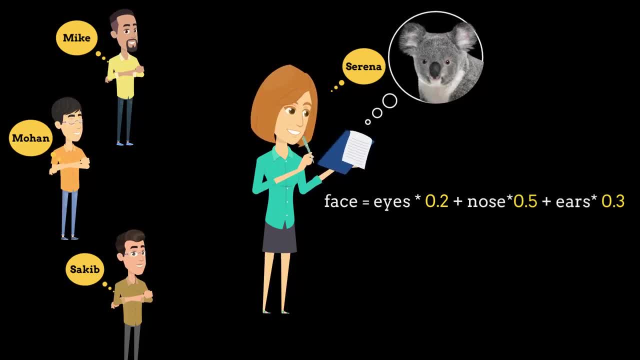 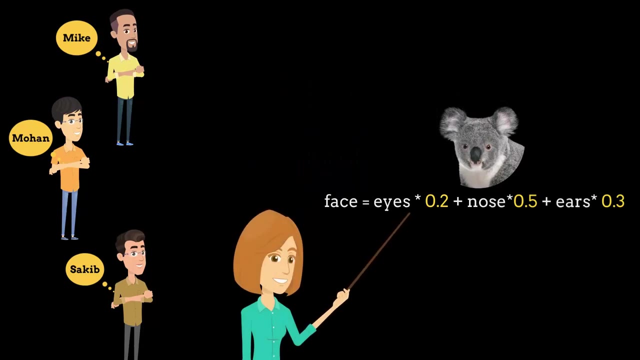 because if you look at koala, the nose in koala is very prominent. Koala's nose are very different than other animals, So if there is a prominent feature, then you can give that more. based on her weight- And Serena can derive this formula for detecting the face- And based on the 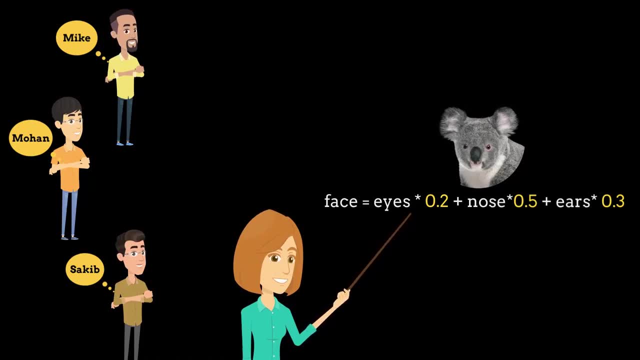 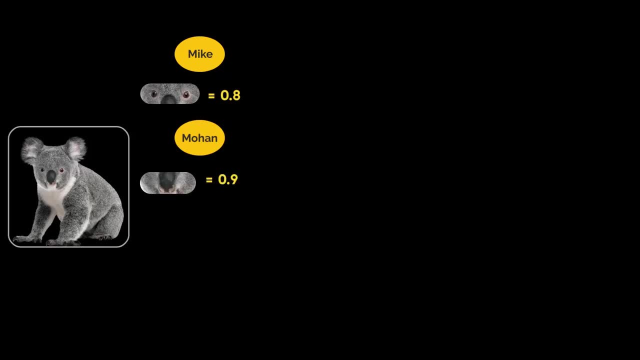 scores that Mike, Mohan and Shakib gives. She will simply use this formula and tell you whether the image has koala's face or not, For example. in this particular case, I have given sample scores by each individual person and Serena computes the phase score to be 0.79. 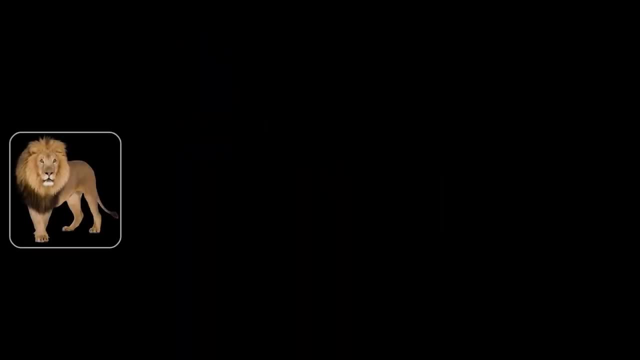 So if anything is more than 0.5. It means it is Koala's face. Similarly, if there is lion's image, you will see that, based on the score, the face score will be 0.15, which means it it is remotely looking. 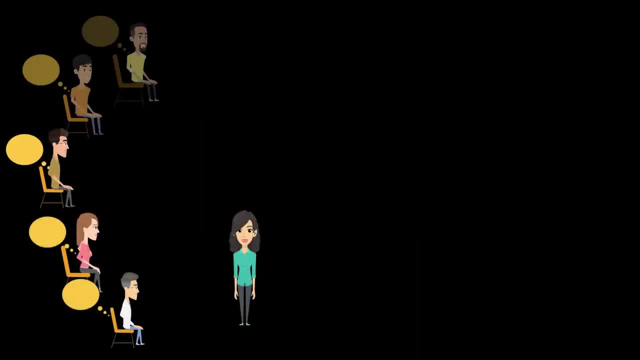 like Koala's face. here You can now use rest of the group where they individually- for example Jyoti can detect legs and Chen can detect tail, and they can tell that decision to Nidhi, whose job is to say whether the image has Koala's body. 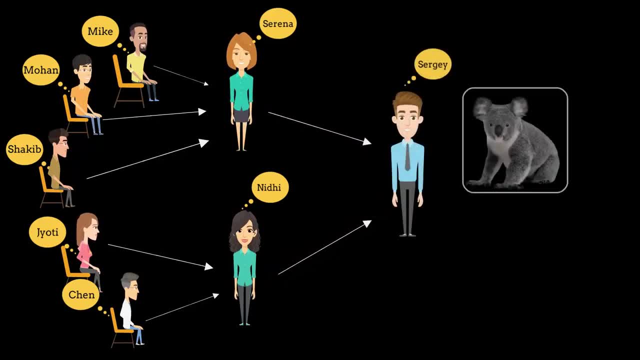 or not. And finally, Serena n SIM and Nidhi will go to Sarge, who will give the final answer and he will also use some kind of formula. here I am giving more weightage to face, because when we are working on face detection- either humans or animals, you know when we are working on. 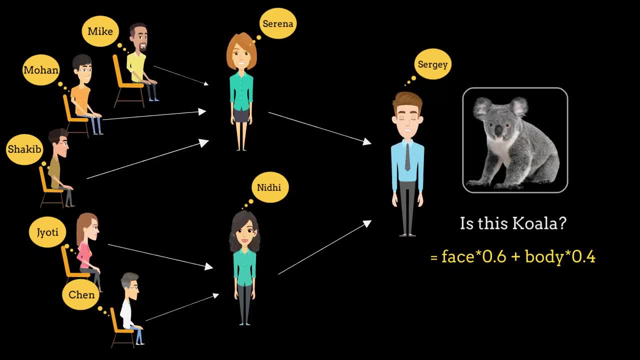 detection adolescence, we will still have to significant amount of weight that we will should have to determine. that will determine if we can guessed honestly the whether it has humans or which animal we give more weightage to face. So now this group is doing this awesome teamwork and telling you whether the given image is. 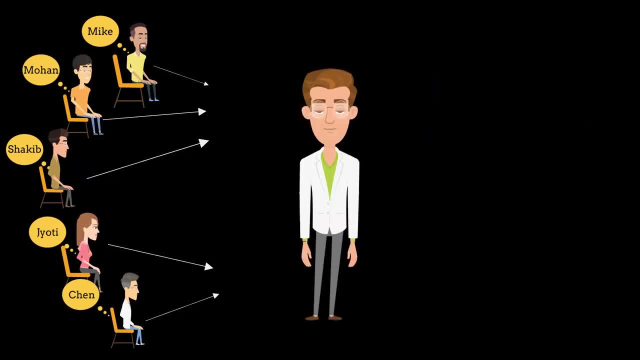 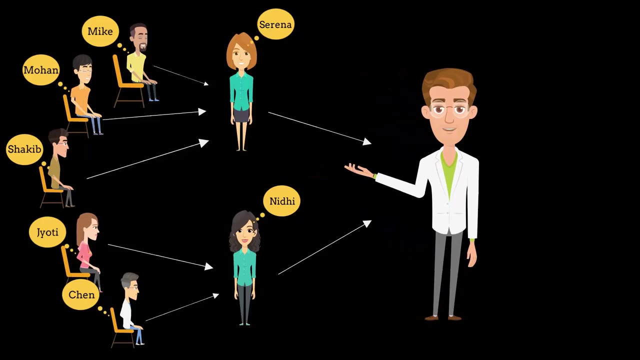 koalas image or not, This is nothing but a neural network. Each individual person here are individual neurons and they are working on a specific subtask and they pass the result of their subtask to the next group. So Serena and Nidhi are 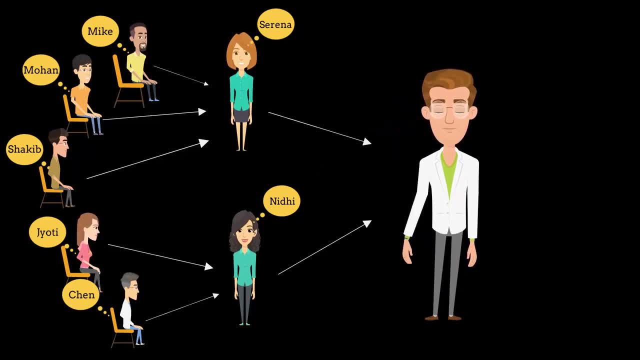 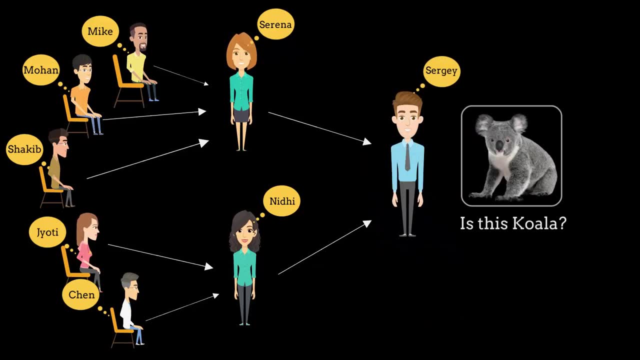 actually, in terms of neural network, they are a hidden layer: Mike, Mohan, etc. they are forming the input, or the first layer, and Sergei is the output or the last layer. So this is a neural network. It's a trained neural network. Now the most. 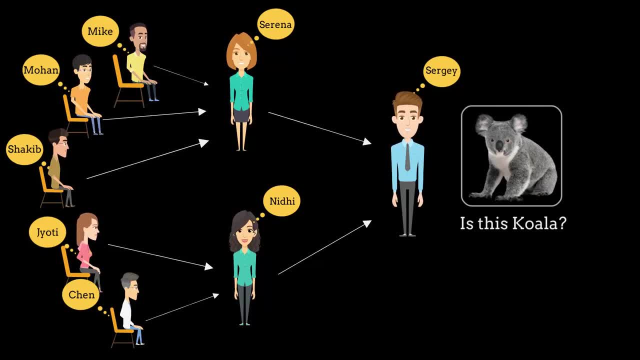 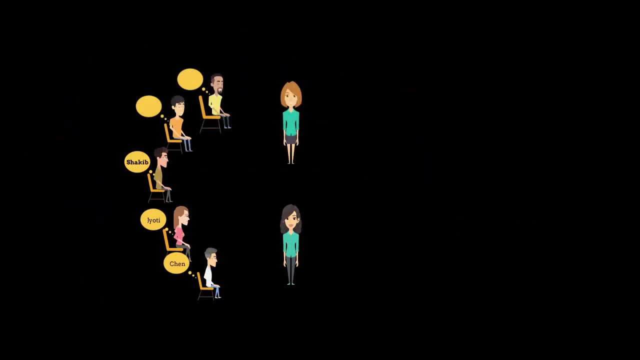 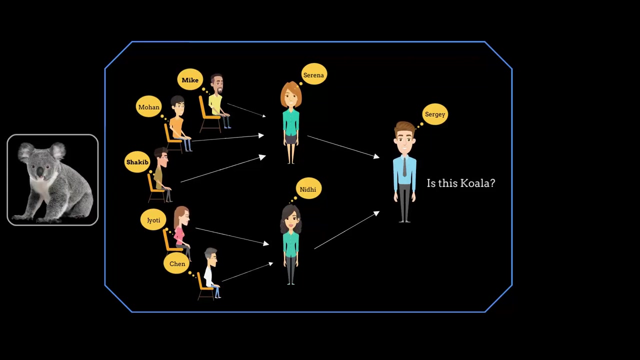 important thing about neural network is how do you train it and how do you detect these features. So just imagine that these students are not trained right now. You put all of them in a classroom and then you supply an image to this classroom and they will. 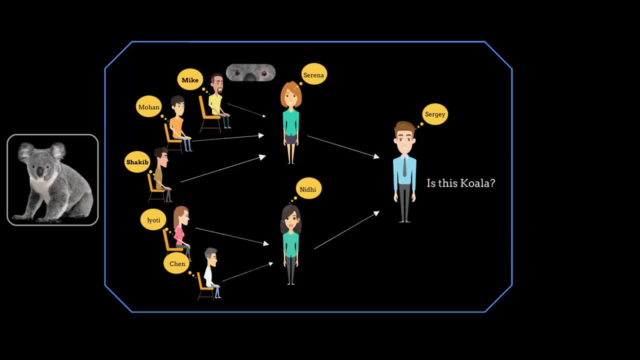 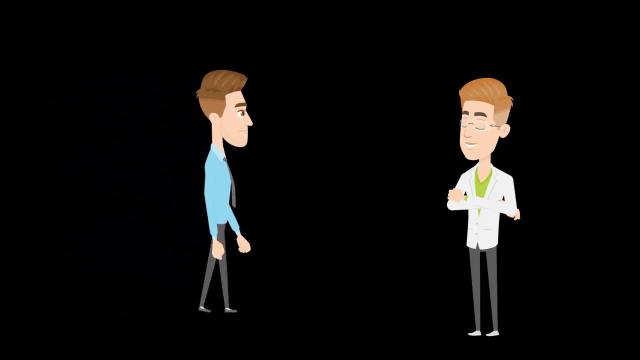 initially make a random guess. So Mike will randomly guess whether this image has koalas eyes or not, and similarly, everyone will make a random guess and finally Sergei will tell whether this is koala or not. And once Sergei has a decision, he will go out out of the classroom and there is a supervisor who 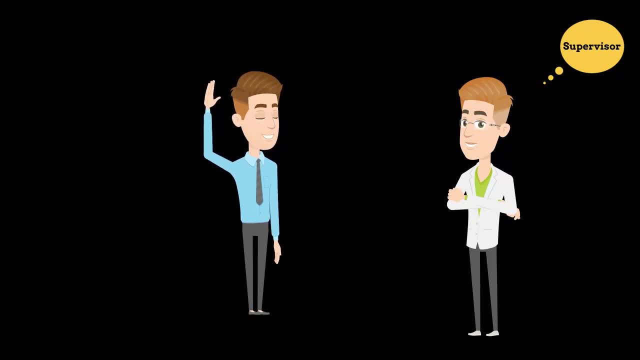 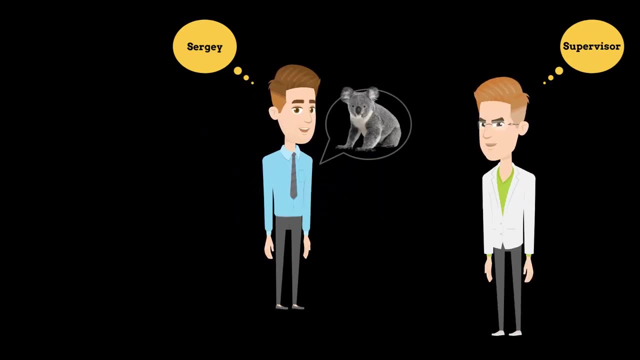 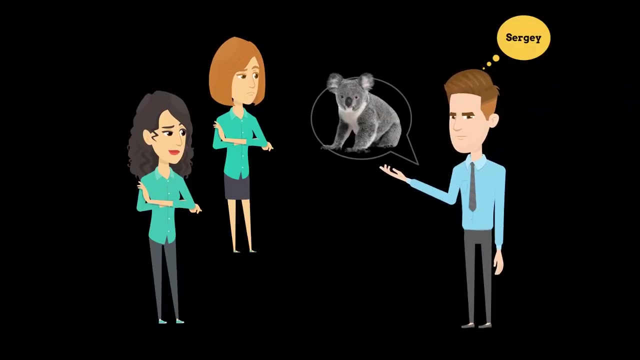 is standing. The supervisor knows the correct answer. So Sergei will say: hello, sir, this doesn't look like koala. and supervisor will be like: no, you're wrong, this is koala. Sergei then goes back to the classroom and says: hey guys, this is actually koala. what score did you give me? Serena? and Nidhi will then go back to. 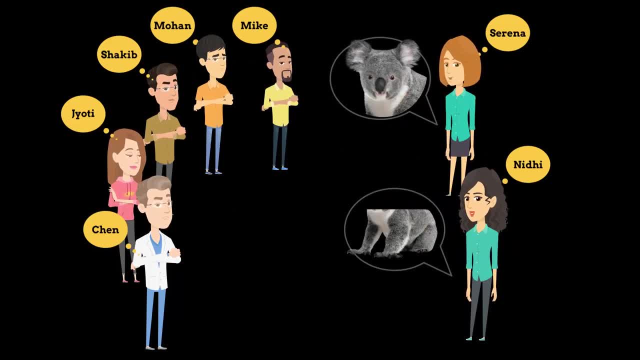 rest of the classroom and say: hey, Mike Mohan Sakib, this is actually koalas ears, eyes and nose. You need to be careful next time. So they use this experience of mistake. So, basically, as a group, they made a mistake and the mistake, or the 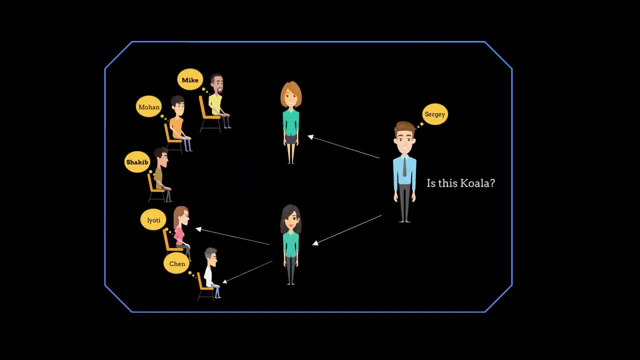 error has been passed from Sergei to Serena Nidhi to rest of the group. This process is called backward error propagation. So you make a mistake and then you get the feedback that you have made a mistake and you pass this feedback to rest of the group so that they adjust their weights. 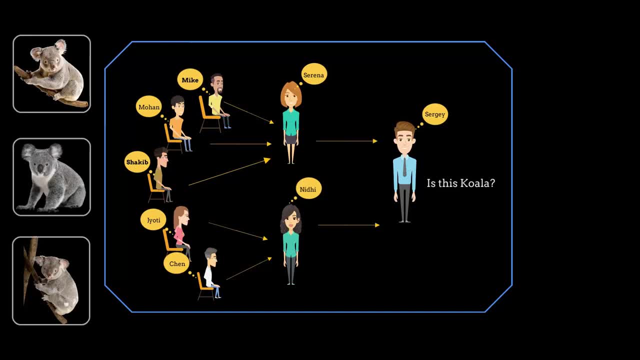 You can take n number of koalas images and repeat the same process. So the same process is repeated, where you make a random guess. then Sergey goes out and tells the supervisor that this is koala or not. The supervisor will tell you if the answer is correct or not and the error feedback is: 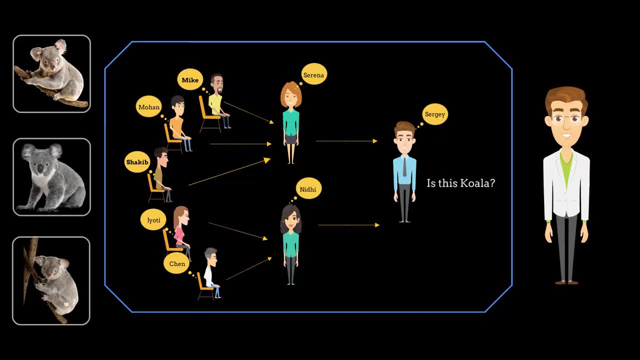 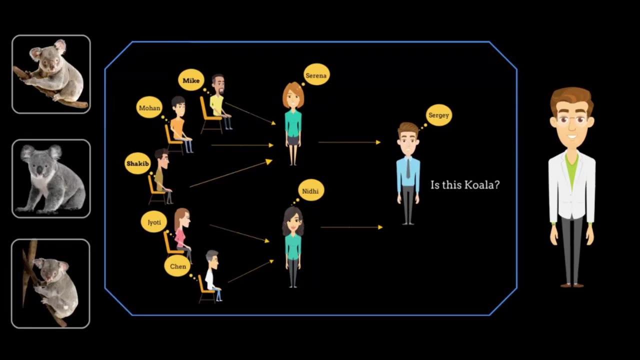 passed on to rest of the group and the group keeps on adjusting their weights or adjusting their brains in a way that they can finally come up with the right answer. You can be given thousands or ten thousand such koalas images and after training this group for so many images, eventually the group becomes better at koalas failure. 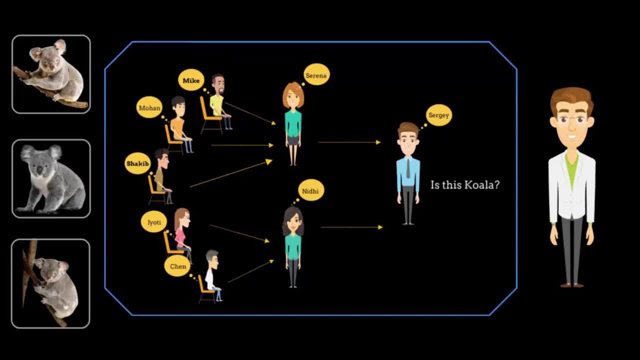 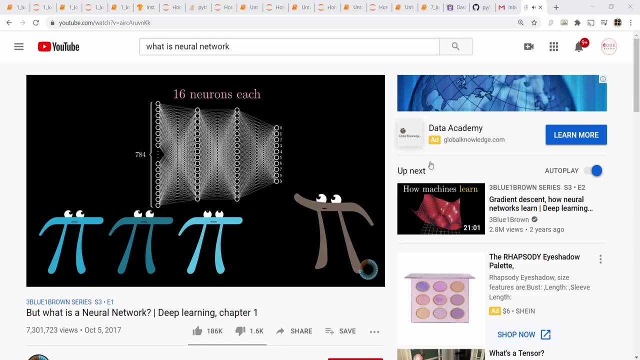 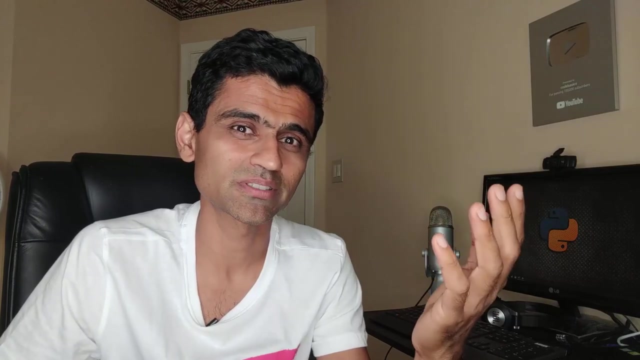 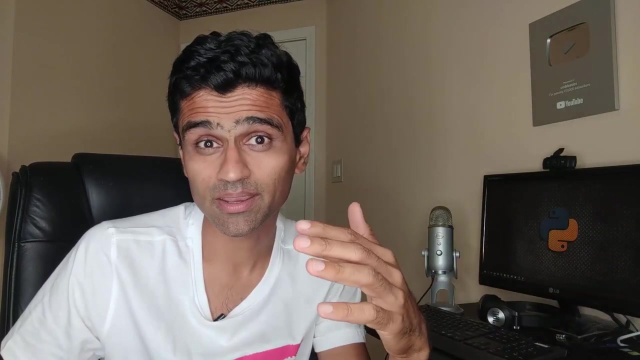 The motivation behind neural networks came from the way human brain works. If you remember those days when, as a kid, you were trying to learn bicycle, you would initially fall down. then you try again, again, fall down, try again and eventually you master that skill. 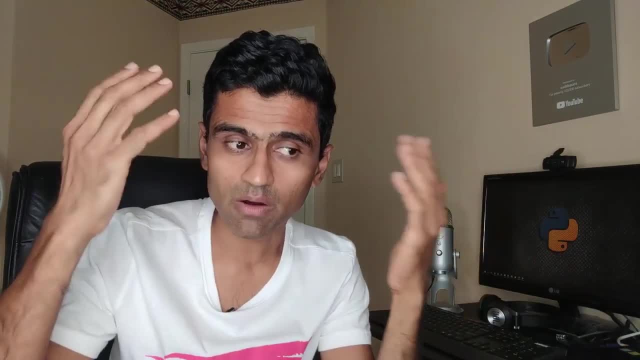 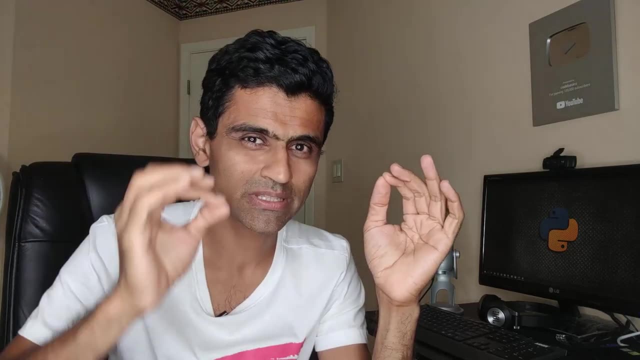 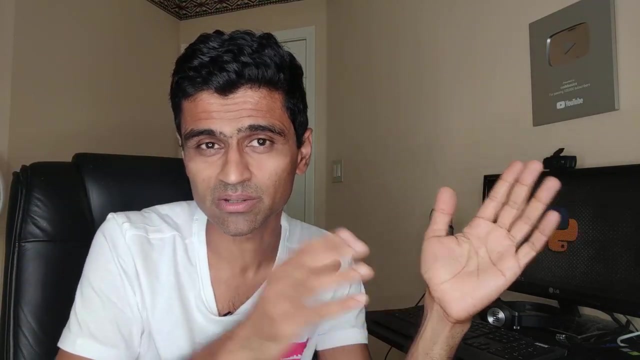 During those trial and errors, what's happening is our brain has billions and maybe trillions of neurons and in those neurons this training process is constantly going on. So there is this error loop, or a back propagation feedback That goes inside those tiny neurons and the weights between those neurons are constantly. 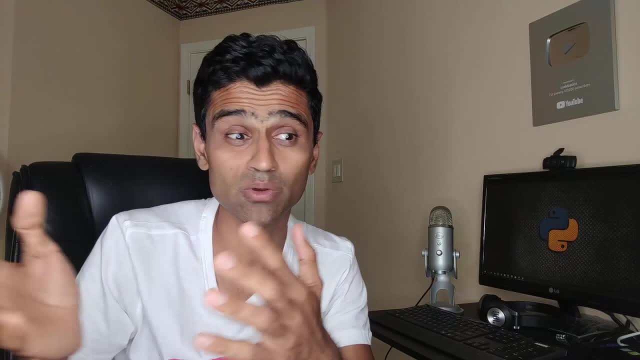 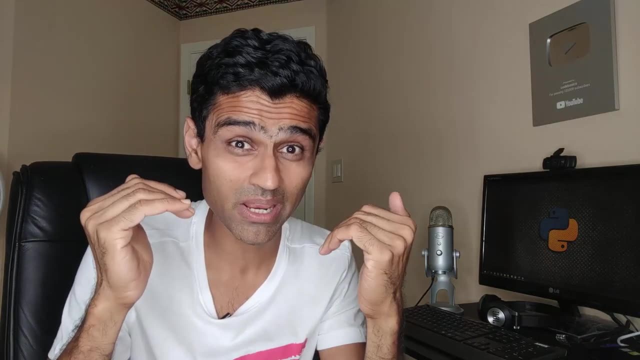 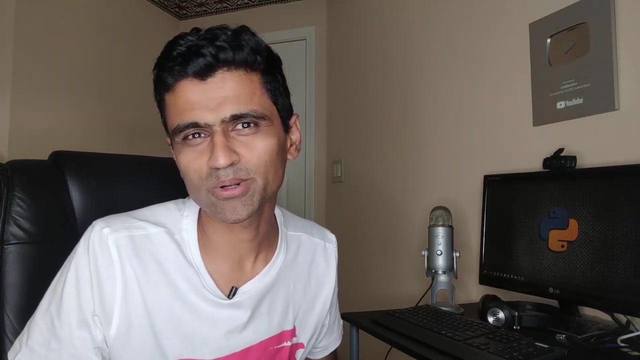 being adjusted until you get into a situation where you are making minimum amount of mistake. Right now, when you are learning deep learning, actually, inside your brain there is a deep learning going on. Isn't that amazing If you have little software engineering background and if you reflect on our previous presentation? 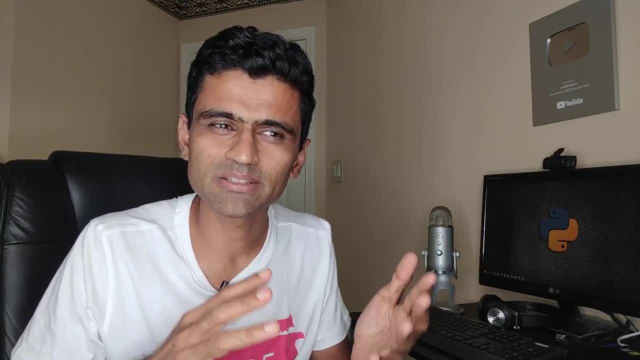 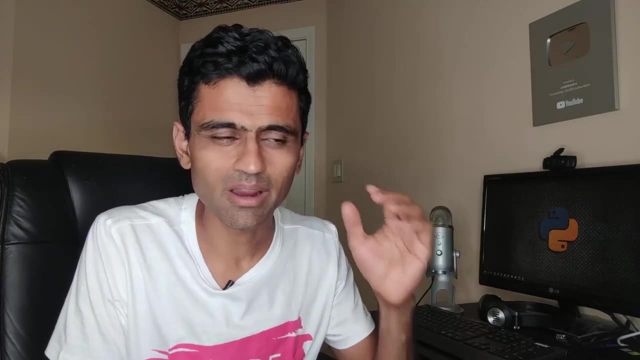 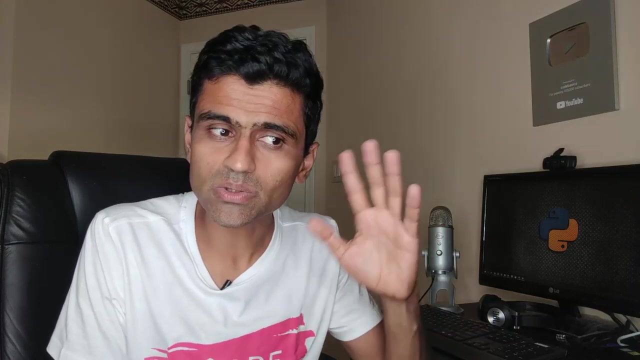 on koalas image detection. You might argue that This looks more like a distributed computing, where each individual person- Mike, Mohan, Seryan, etc. are working on a well-defined task and their results are being aggregated at the later stage. 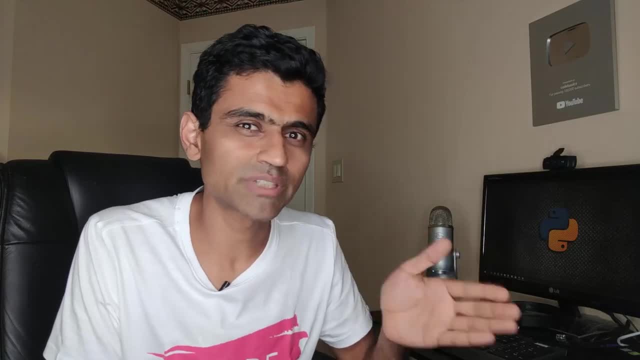 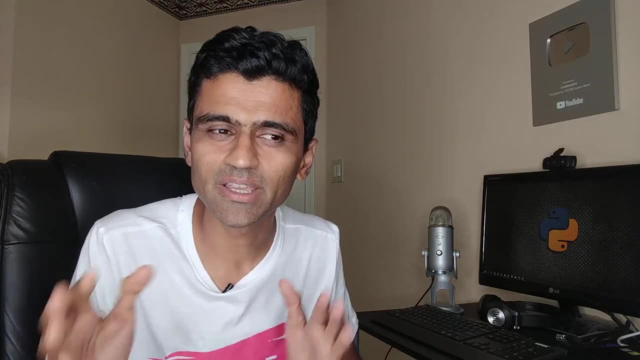 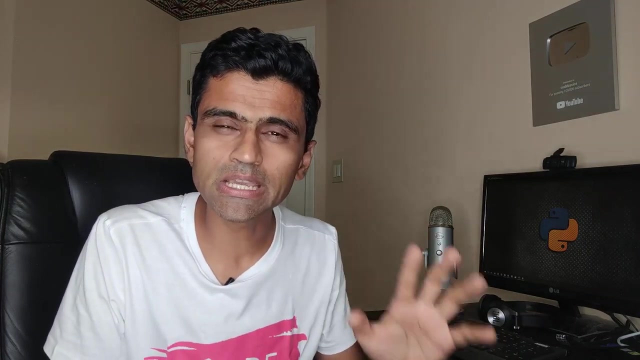 And it is okay to think that way. But that is not the most interesting part about neural network. The most fascinating aspect about neural network is the training itself. Imagine that you are not telling each individual students what they should be working on, And these guys, although they are naïves, they figure out in a smart way what exact. 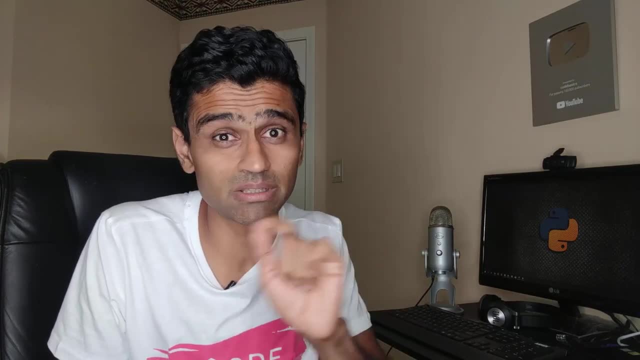 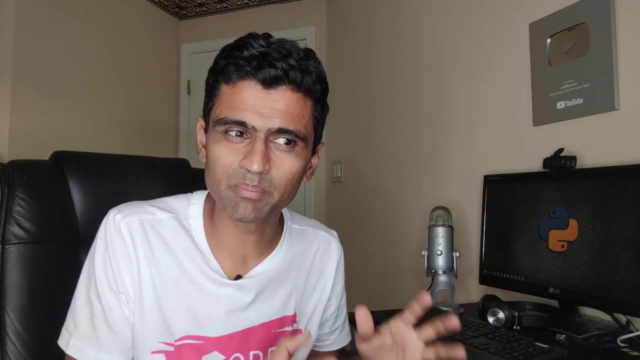 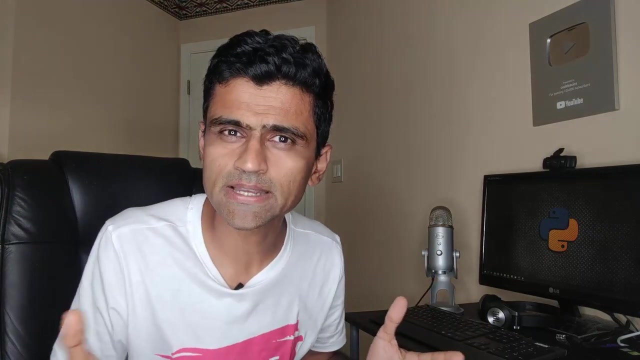 sub tasks they need to work on or what exact feature they need to work on. That is the most interesting part about neural network, And there is a mathematics involved behind that, which we'll look into it in a later video. But in the real life, when you are dealing with a complex data sets you do not know. 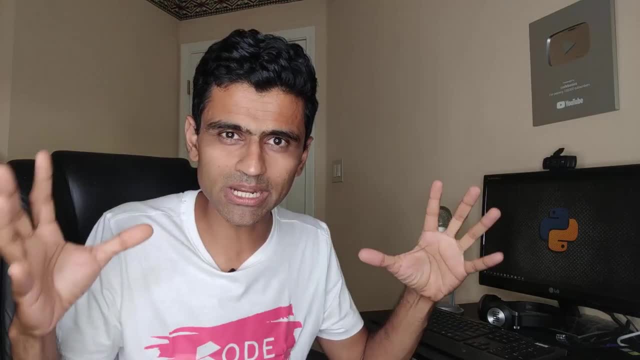 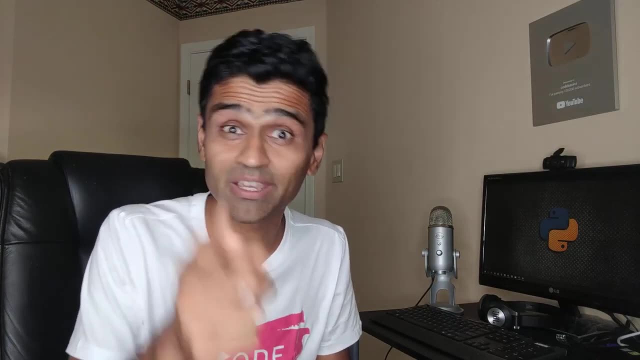 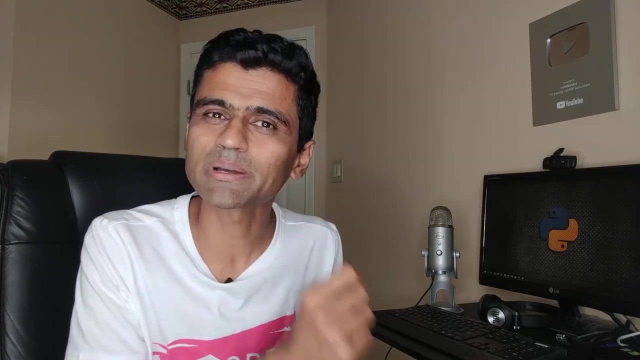 what features you are looking at. So you just build a neural network which has input layer, a couple of hidden layers and the output layer, and neural network will figure it out for you. So each individual neurons are so smart that they will figure out what sub tasks they need. 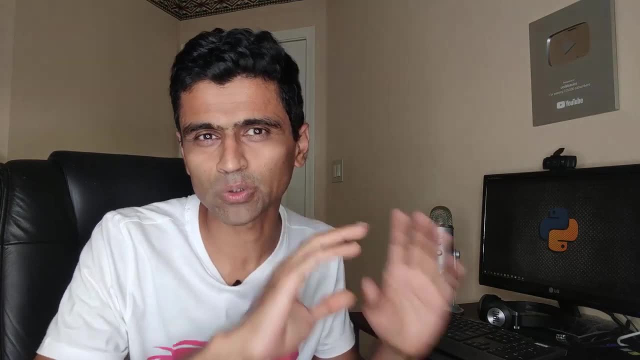 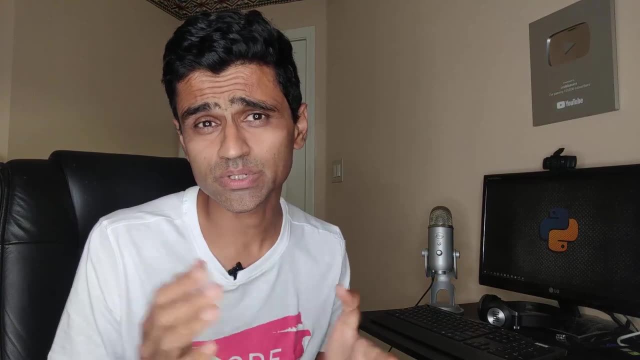 to work on. All you need to do is you need to give a lot of truth data to it. I hope that clarifies some of the doubts that you had about neural network. If you like this video, please post in a video comment below. 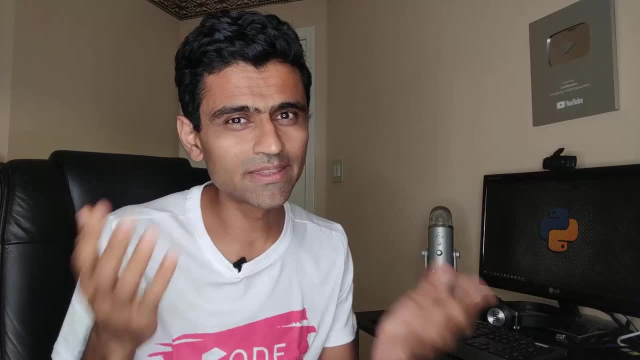 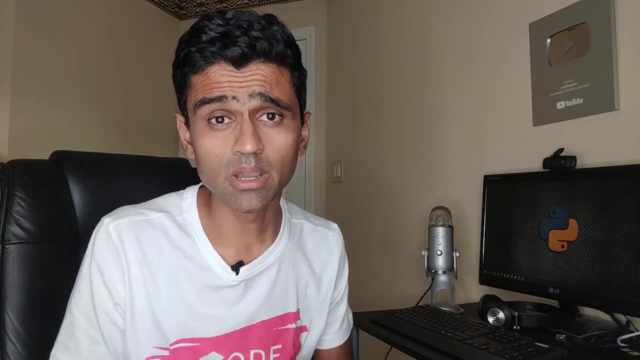 That way, You can give feedback on the content that I'm producing. in this deep learning tutorial series, I'm going to demystify many different concepts in deep learning world, such as convolutional neural network, RNN, activation function and so on. 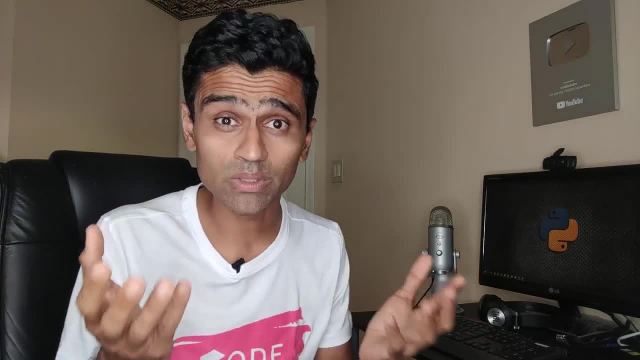 And we'll be writing Python code using TensorFlow along with the exercises. Thank you for watching. I will see you in the next video.